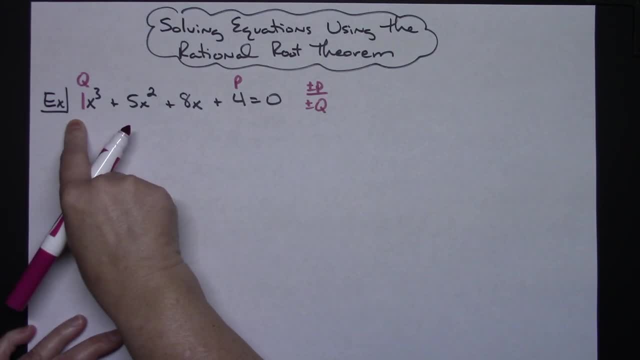 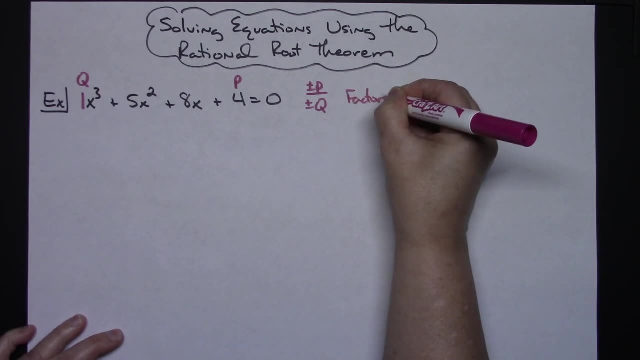 So we're going to be putting all of our factors of p over one, so there's not going to be a lot there to test, So. So basically, I've got to look at my factors of plus or minus one, plus or minus two and plus or minus four. 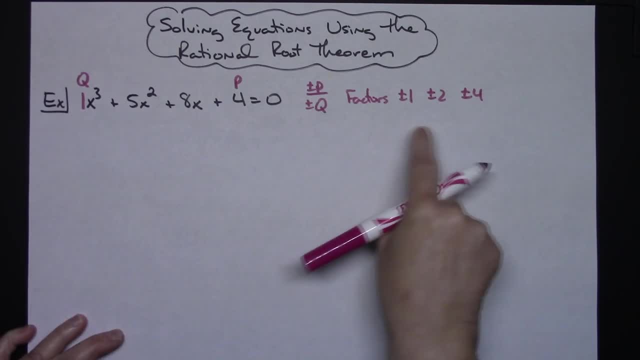 Because it would be four. you know all the factors of four. you know p over q. So you're going to then take a look at these and really, in all honesty, you're just going to pick one. You're going to pick one and do synthetic division over and over and over until you get one that works. 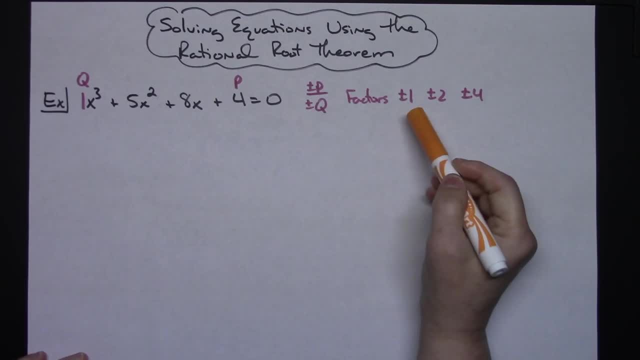 Okay, so let's just start. Normally, I will start with a plus or minus one. I usually don't start with the larger numbers, But I definitely want to get one that doesn't work, to show you what happens, what you have to do when it doesn't work. 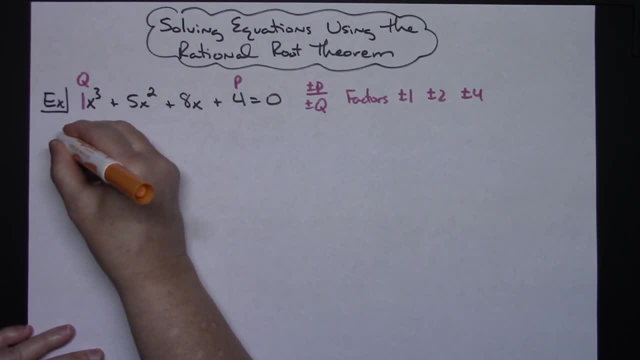 Alright, so let's say you decide you want to try four there, So I'm going to do my four and then I'm going to do synthetic division. So I'm going to take all those coefficients there and I'm going to have a one and a five and an eight and a four. 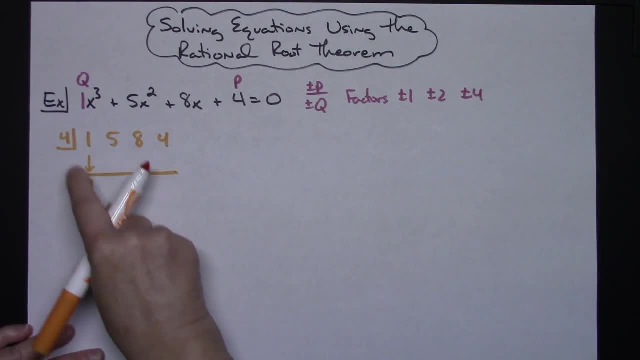 I'm going to bring that one straight down. One times four is going to give me a four. Alright, we always add going down. That would be nine. Nine times four is thirty-six. Again, adding going down, that's going to be like forty-four. 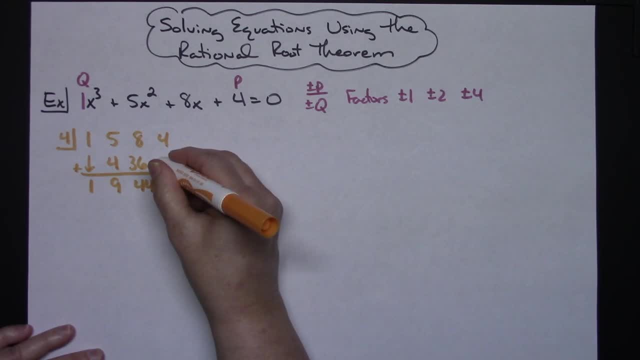 And then forty-four times four, one hundred and seventy-six, if I'm not mistaken. That one even could be wrong, But regardless, when I add going down here, I am not going to get a zero, which is what I need. 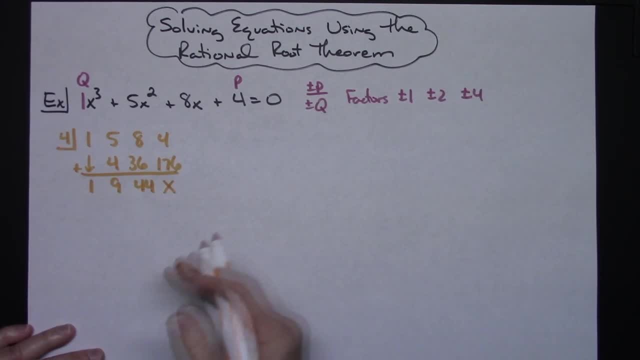 So this doesn't work, Okay, so you try one. it doesn't work, Then you try another number for your list, Okay, and so forth and so on. So I don't know, let's try, say two. 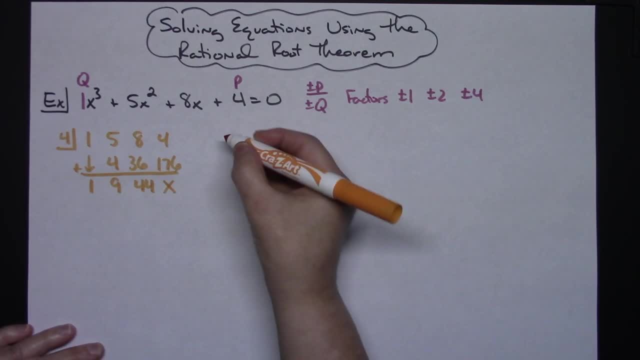 Okay, so I could put: then let's do a negative two, Let's put a negative two in our box right there And then do our coefficients. So one, five, eight and four, Bringing down that one One times a negative two is a negative two. 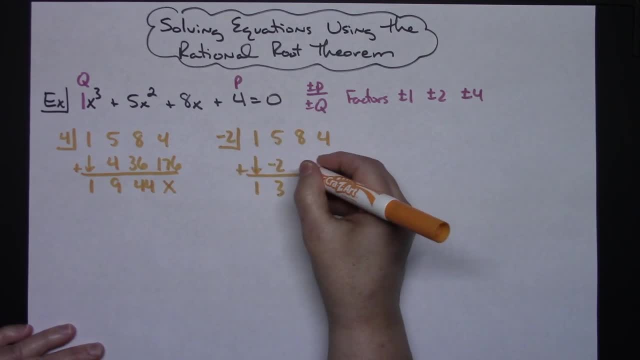 Add going down, I'm going to get a three. Three times negative two will give me a negative six. Add going down: I get a two, Two times that negative two will give me a negative four. Four plus negative four gives me a zero. 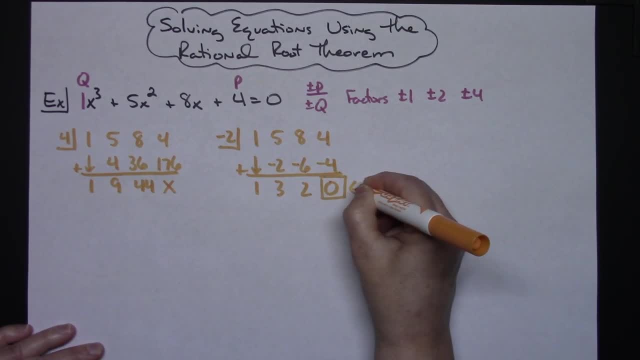 And that is what I need. I need a remainder of zero. Okay, and the thing is, the reason I wanted to do one that wasn't going to work out, because not every one of those numbers are going to be a factor. Okay, so you're not always going to get a remainder of zero. 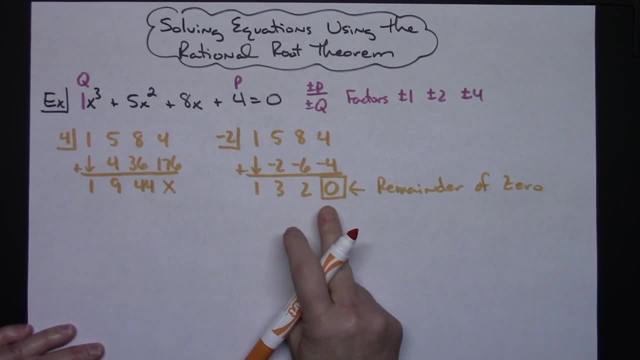 So you have to, in theory, try several of them until you find one that comes up with that remainder of zero. But once you do that, then what this does is it takes this four terms and gives you the factored form of that. 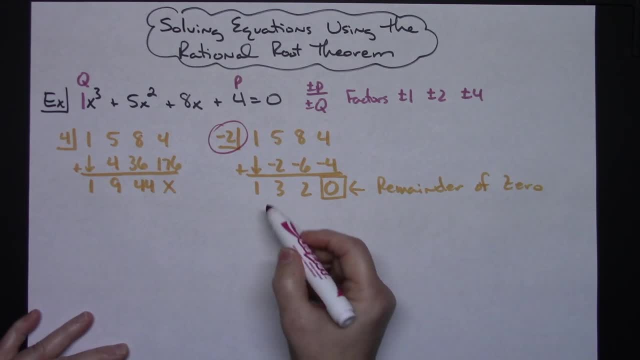 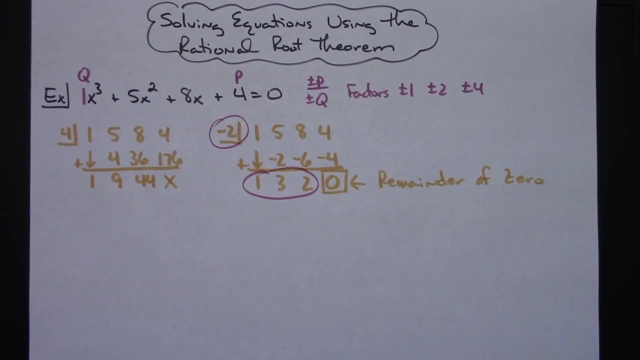 Because you're going to use this to come up with a factor, because you know that's a factor And you know this is what's left over. Alright, now let's come and actually write all of this out. So I'm going to start with that original four terms. 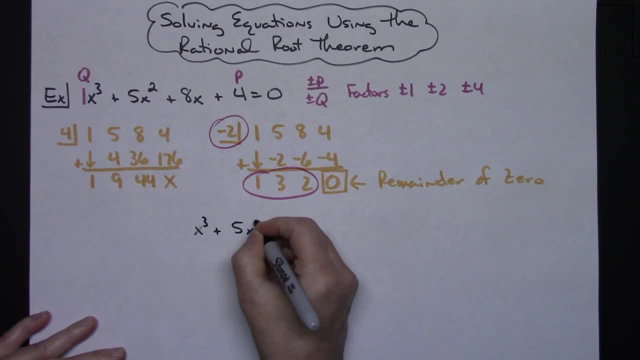 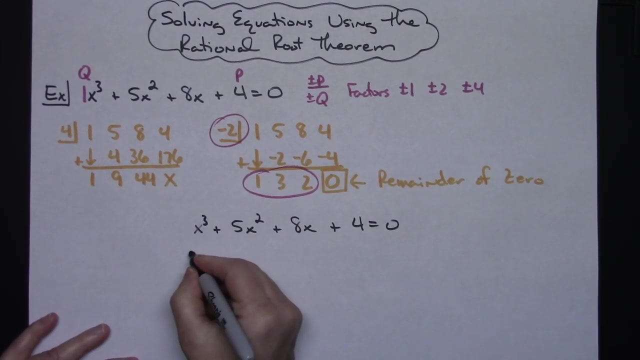 X to the third Plus five, X squared Plus eight, X Plus four Equals zero. Alright, now I'm going to get a factor from here. If negative two goes into this with a remainder of zero, I know two X plus two has to be a factor. 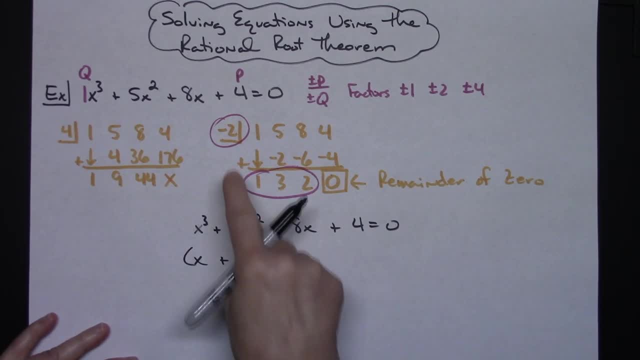 So I'm going to write it as X plus two. Alright, now this divides into this four terms. with this as our remainder, We're going to take this and write it as I mean. that's your remainder. This is what's left over. 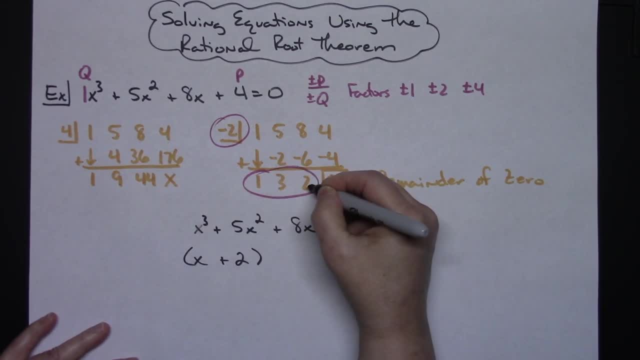 I'm going to write this as a trinomial, So this will be my plain number, This will be my X, And then this will be my X squared. So from here I can write the trinomial X squared plus three, X plus two. 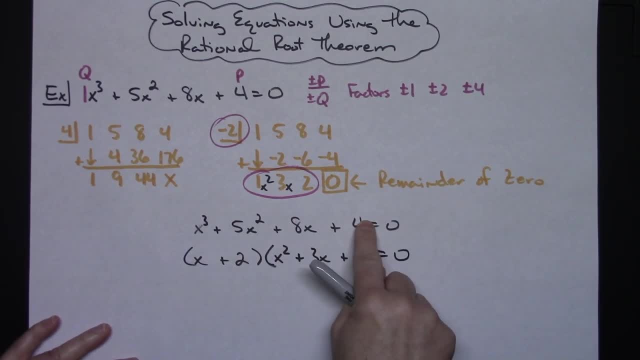 Alright, these two things multiplied together will equal this polynomial of four terms. Alright, you could check that by FOILing that out and checking: Alright, now this term has already been factored. Hopefully this will work. This is going to give you a trinomial that you can factor by hand. 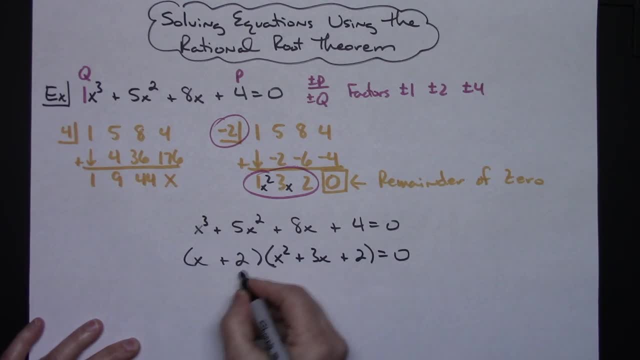 This one is going to factor into a two and a one, which it is going to work. So this term right here, X plus two, is going to stay. This trinomial will factor into an X and an X. We're going to use a two and a one, with pluses there.